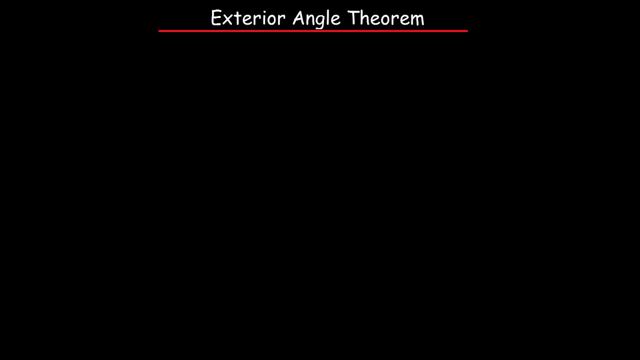 In this lesson we're going to talk about the exterior angle theorem, That is, the exterior angle of a triangle is the sum of the two remote interior angles. So let's use an example to illustrate this. So here's a triangle. Let's do that again. 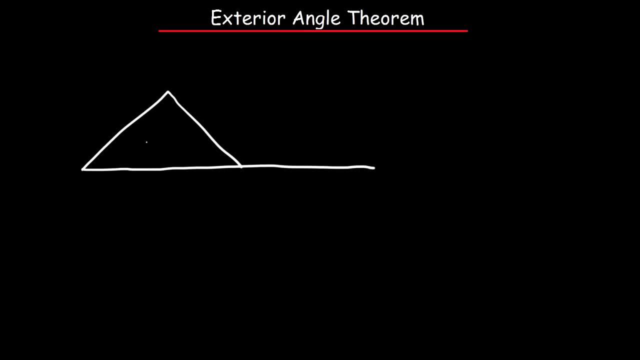 And let's say this angle is 40 and this angle is 60. What is the value of this angle? Now, before we find the answer, let's call this angle 1,, 2,, 3, and 4.. Angle 4 is outside of the triangle, So it's the exterior angle. Exterior means it's on the outside. 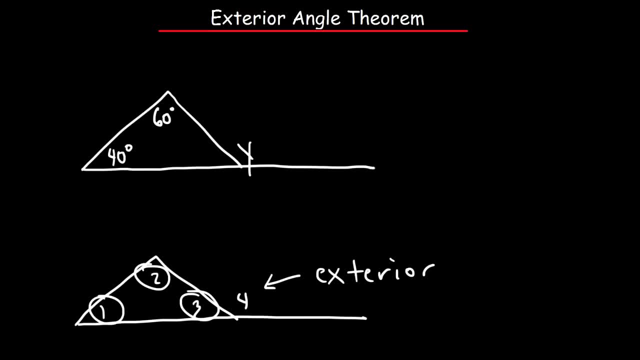 Angles 1,, 2, and 3 are the interior angles because they're inside of the triangle. However, 1 and 2 are known as the remote interior angles And 3 is just an interior angle. So the exterior angle, number 4, is the sum of the remote interior angles. That's the sum of angle 1 and 2.. 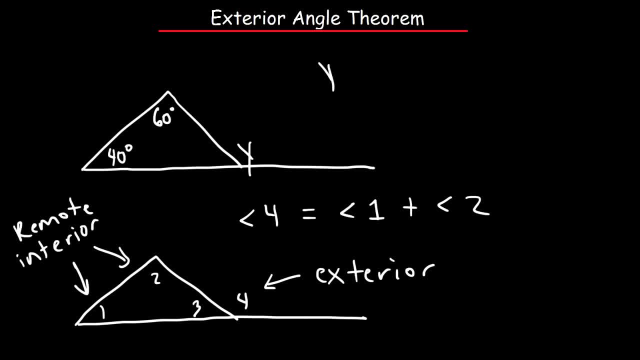 And we can say that y, the exterior angle, is the sum of these two remote interior angles, 40 plus 60. And so y is 100 degrees. Now we know that the three angles in a triangle must add up to 180.. So if we call this x, we can say that x plus 40 plus 60 has to add up to 180.. 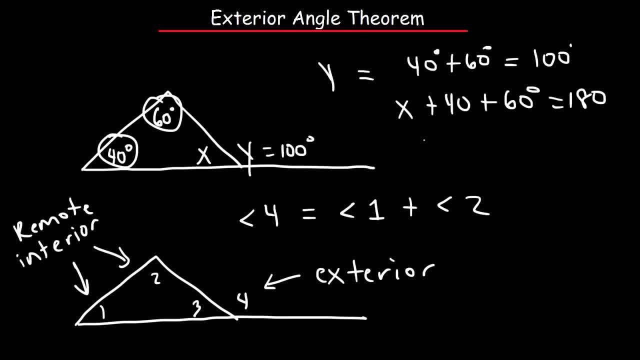 40 plus 60 is 100.. And 180 minus 100 is 80.. So x is 80.. Now notice that these two they form a linear pair. So x plus y adds up to 180.. 80 plus 100 is 180.. 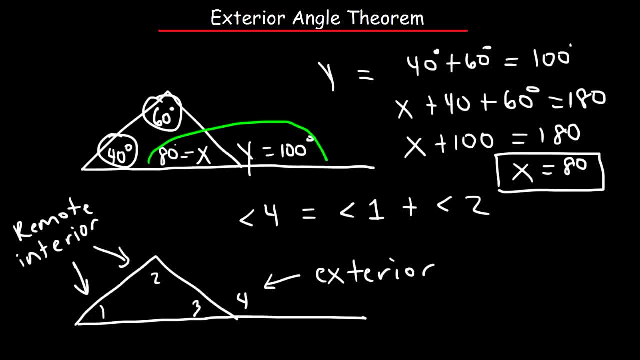 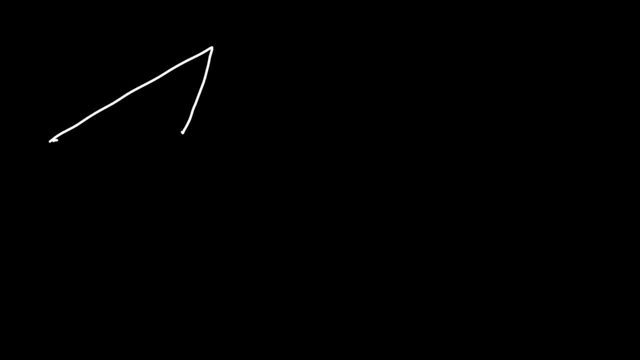 Anytime you have a linear pair it always adds up to 180.. So let's work on some other example problems. So let's say: if this is 40,, this is x, and let's say this is 110, and this is y. 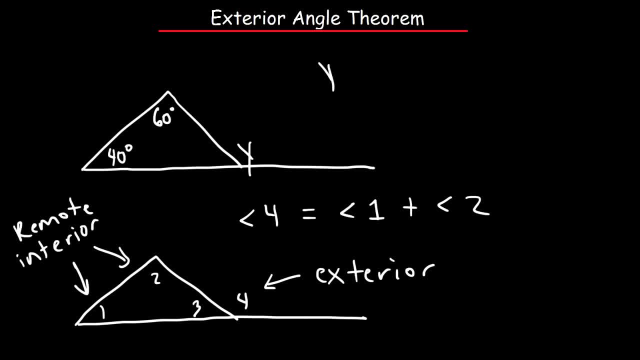 And we can say that y, the exterior angle, is the sum of these two remote interior angles, 40 plus 60. And so y is 100 degrees. Now we know that the three angles in a triangle must add up to 180.. So if we call this x, we can say that x plus 40 plus 60 has to add up to 180.. 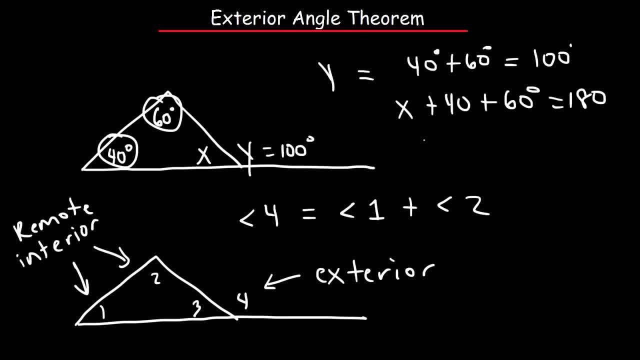 40 plus 60 is 100.. And 180 minus 100 is 80.. So x is 80.. Now notice that these two they form a linear pair. So x plus y adds up to 180.. 80 plus 100 is 180.. 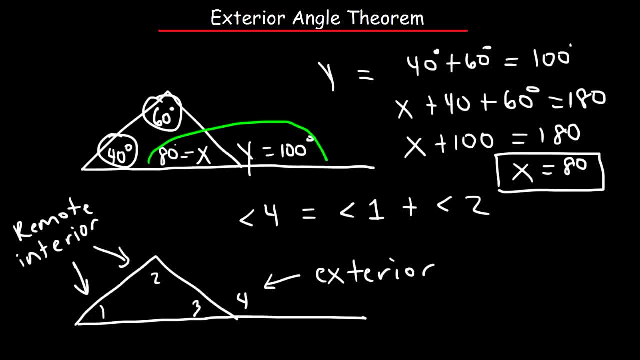 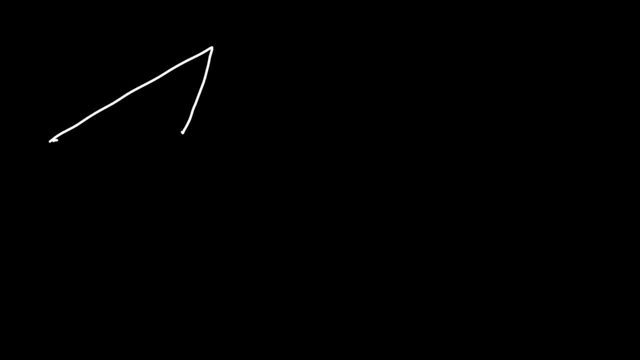 Anytime you have a linear pair it always adds up to 180.. So let's work on some other example problems. So let's say: if this is 40,, this is x, and let's say this is 110, and this is y. 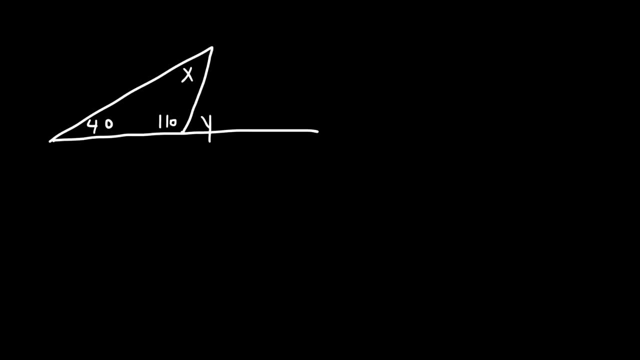 Calculate the value of x and y. Feel free to pause the video. So we know that y, the exterior angle, is the sum of the remote interior angles. So we can say that y is 40 plus x And also notice that 110 and y- they form a linear pair, so they add up to 180. 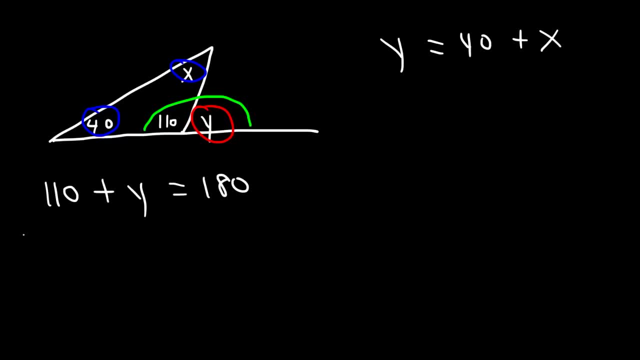 So we can easily find the value of y. So if we subtract both sides by 110, we can see that y is 180 minus 180. So we can say that y is 110, or 70 degrees. Now with that we can calculate the value of x. 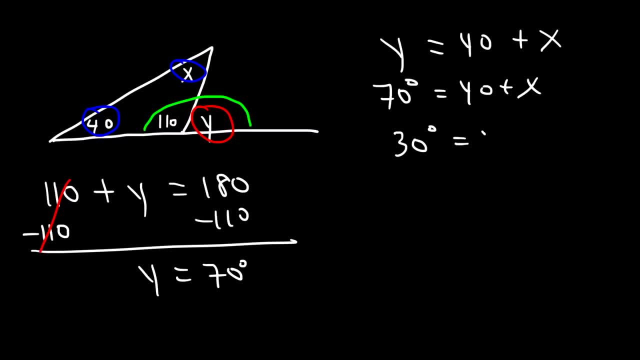 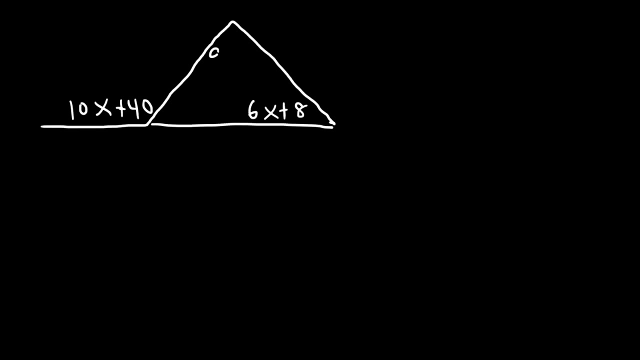 So 70 minus 40 is 30. So x is equal to 30 degrees. Let's try another example. So let's say this is 10x plus 40. And let's say that here we have 60x, 6x plus 8.. 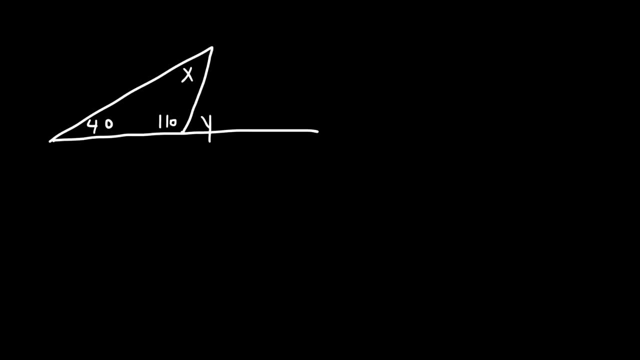 Calculate the value of x and y. Feel free to pause the video. So we know that y, the exterior angle, is the sum of the remote interior angles. So we can say that y is 40 plus x And also notice that 110 and y- they form a linear pair, so they add up to 180. 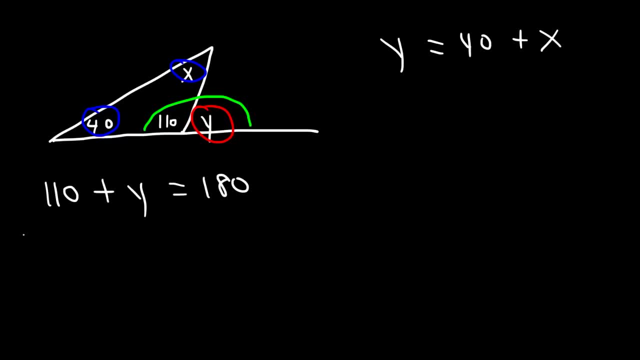 So we can easily find the value of y. So if we subtract both sides by 110, we can see that y is 180 minus 180. So we can say that y is 110, or 70 degrees. Now with that we can calculate the value of x. 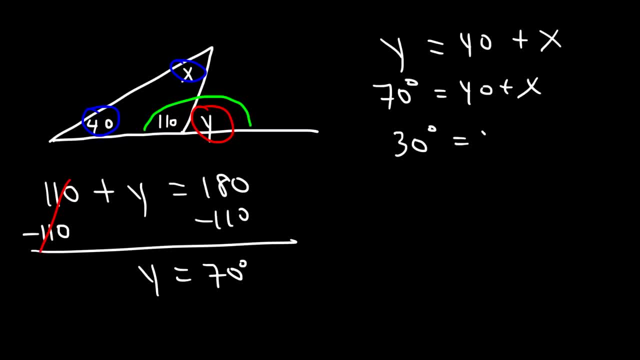 So 70 minus 40 is 30. So x is equal to 30 degrees. Let's try another example. So let's say this is 10x plus 40. And let's say that here we have 60x. 60x plus 40 is 3x. 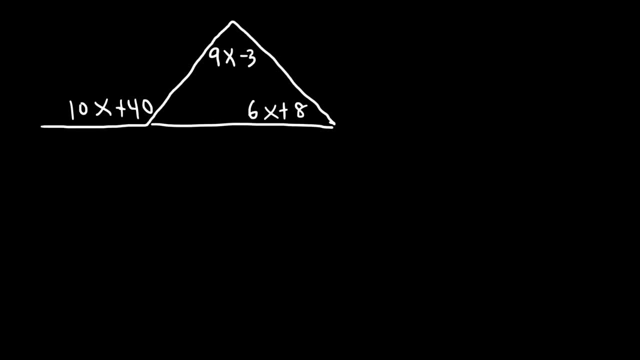 60x minus 40 is 6x plus 8. And this is 9x minus 3.. Now let's call this angle 1,, angle 2, angle 3, and angle 4.. So what I want you to do in this problem is that I want you to first calculate the value of x. 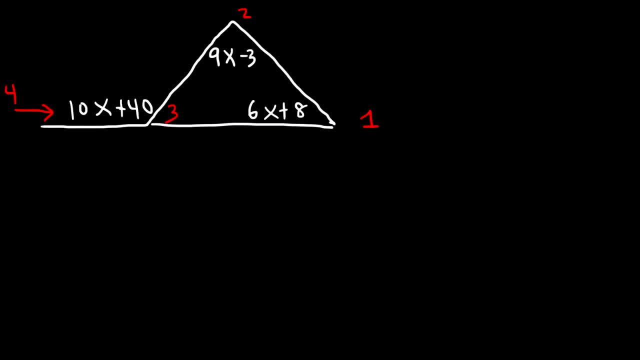 and then use that to find the value of each angle. So go ahead and pause the video and try this problem. the exterior angle is the sum of the remote interior angles. So the exterior angle, 10x plus 40, is the sum of 9x minus 3 and 6x plus 8.. So now let's solve. First let's combine like terms on: 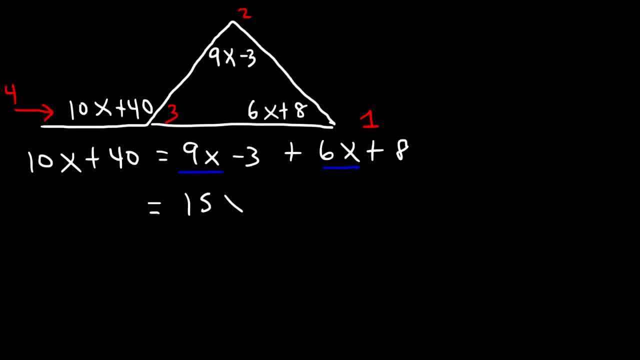 the right side. So 9x plus 6x, that's 15x, and then negative 3 plus 8,, that's positive 5. And on the left we have 10x plus 40. Now let's subtract both sides by 10x And at the same time 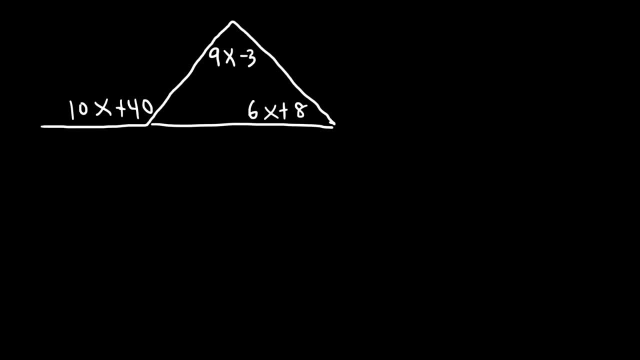 And this is 9x minus 3.. Now let's call this angle 1,, angle 2,, angle 3, and angle 4.. So what I want you to do in this problem is that I want you to first calculate the value of x. 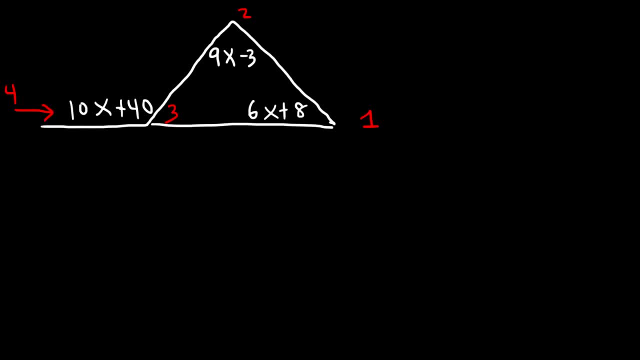 and then use that to find the value of each angle. So go ahead and pause the video and try this problem Now. according to the exterior angle theorem, the exterior angle theorem is the value of x. exterior angle is the sum of the remote interior angles. So the exterior angle 10x plus 40. 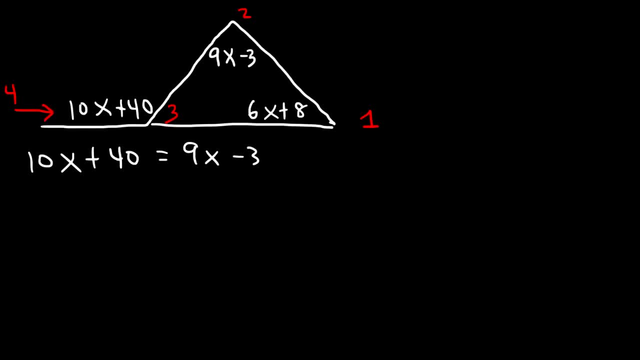 is the sum of 9x minus 3 and 6x plus 8.. So now let's solve. First let's combine like terms on the right side: So 9x plus 6x, that's 15x, and then negative 3 plus 8,, that's positive. 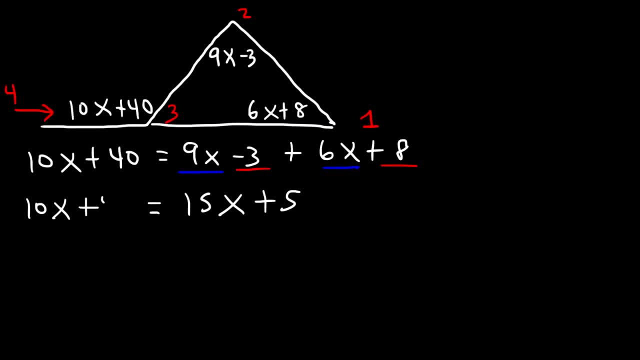 5. And on the left we have 10x plus 40. Now let's subtract both sides by 10x And at the same time let's subtract both sides by 5.. So we cancel these: 40 minus 5 is 35, and 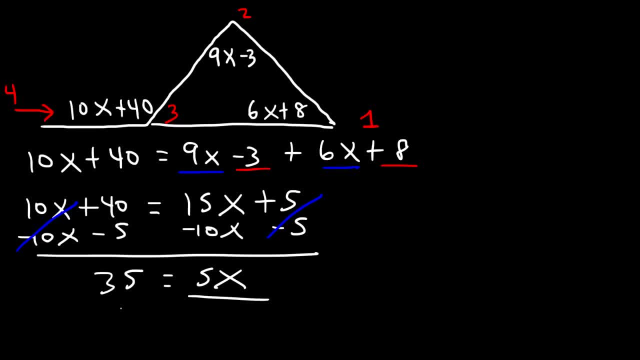 15x minus 10x is 5x. So now let's divide both sides by 5.. 35 divided by 5 is 7.. And so that is the x-axis. So now that we have the value of x, we can calculate the value of each angle. So angle. 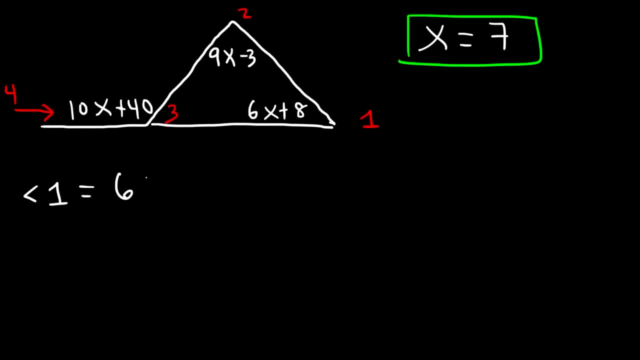 1 is 6x plus 8.. So let's replace x with 7, and let's calculate the value: 6 times 7 is 42, and 42 plus 8 is 50 degrees. So that's the value of angle 1.. Now let's move on to 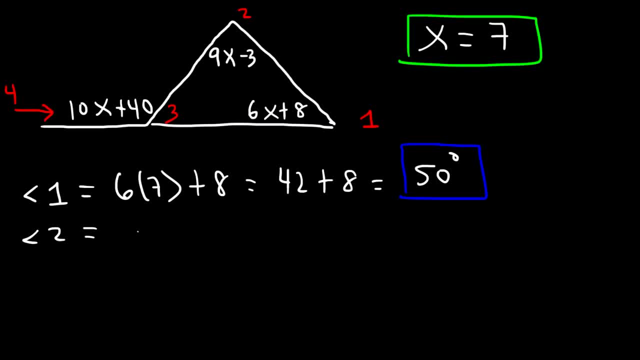 angle 2.. So that's 9x plus 8.. 9x minus 3, so 9 times 7 minus 3.. 9 times 7 is 63.. 63 minus 3 is 60.. Now angle 3.. Notice that angle 1 plus angle 2 plus angle 3 has to add up to 180.. Those 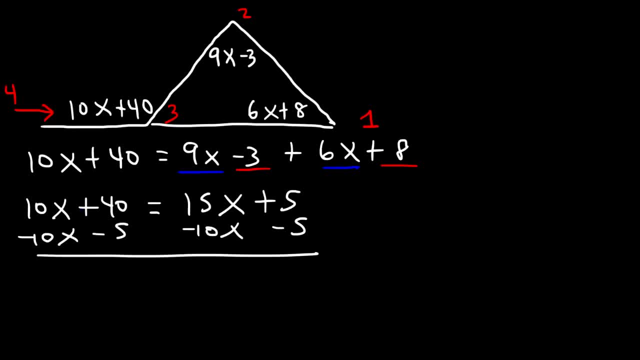 let's subtract both sides by 5.. So we cancel these. 40 minus 5 is 35, and 15x minus 10x is 5x. So now let's divide both sides by 5.. 35 divided by 5 is 7.. And so that is the x value to this problem. 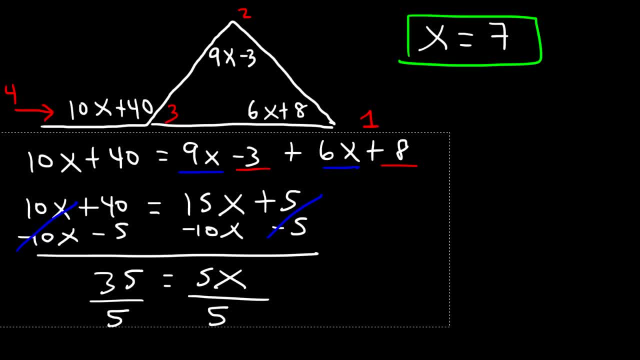 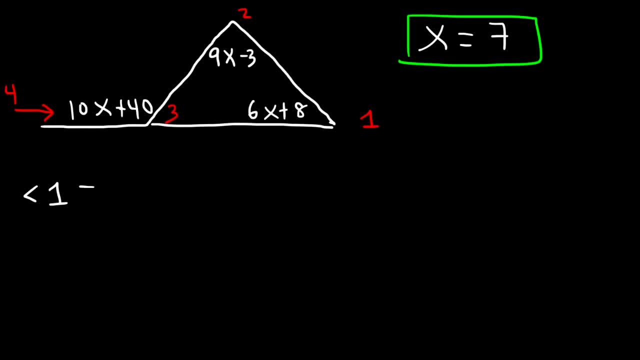 So now that we have the value of x, we can calculate the value of each angle. So angle 1 is 6x plus 8.. So let's replace x with 7. And let's calculate the value: 6 times 7 is 42,. 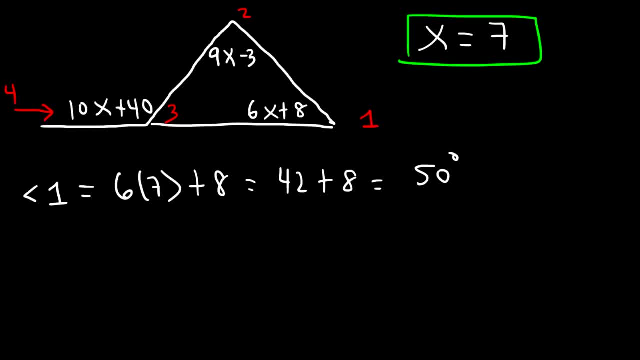 and 42 plus 8 is 50 degrees. So that's the value of angle 1.. Now let's move on to angle 2.. So that's 9x minus 3.. So that's the value of angle 1.. Now let's move on to angle 2.. 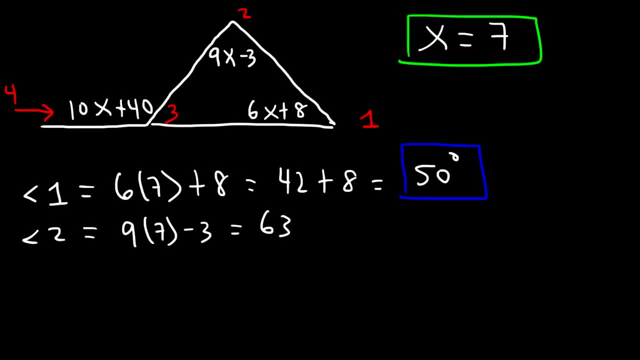 So 9 times 7 minus 3.. 9 times 7 is 63.. 63 minus 3 is 60. Now angle 3.. Notice that angle 1 plus angle 2 plus angle 3 has to add up to 180.. Those are. 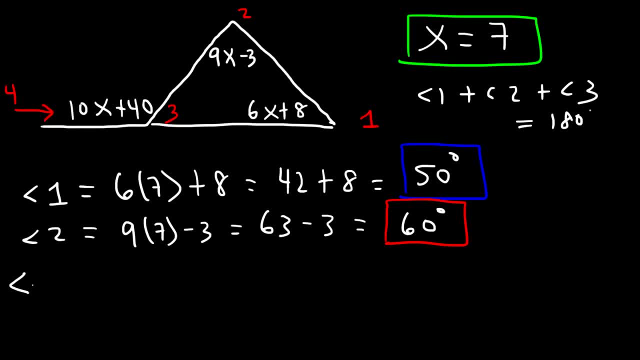 the three angles of the triangle. So angle 3 is going to be 180 minus the other two angles, minus angle 1 and minus angle 2.. So that's 180 minus 50, minus 60.. So 180 minus 50 is 130.. And 130 minus 60 is 70. 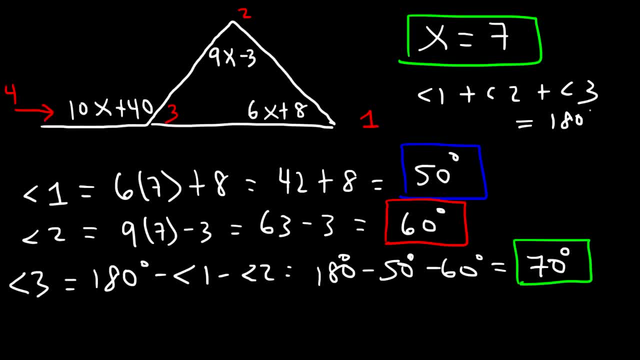 So that's the value of angle 3.. Now angle 4 is 10x plus 40. So that's 10 times 7 plus 40. And 10 times 7 is 70.. 70 plus 40 is 110. And so we can see that angle 4 is the sum of. 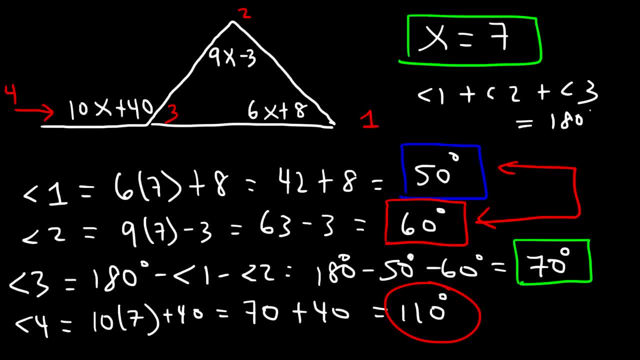 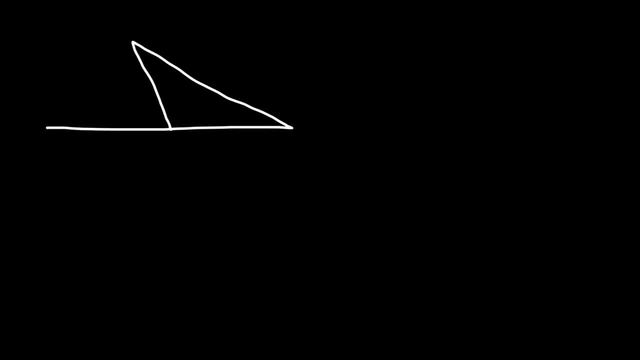 angle 1 and 2.. 50 plus 60 is 110.. Let's work on one more problem. So let's say: let's call this angle A B. let's say this is C and this is D. So angle A, we're going to say it's 8x plus 10.. 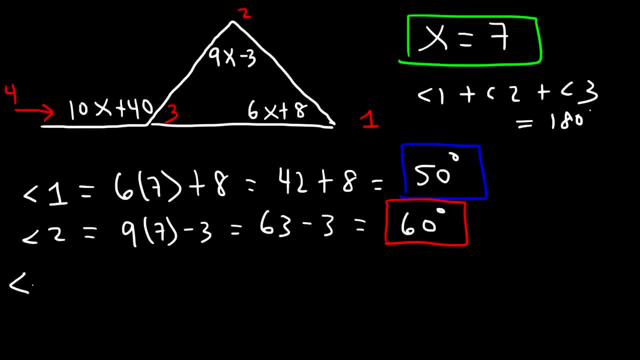 are the three angles of the triangle. So angle 3 is going to be 180, minus the other two angles, minus angle 1 and minus angle 2.. So that's 180.. Now angle 4.. Again angle 4.. Again angle 3 and angle 6.. Forehead angle is the angle that. 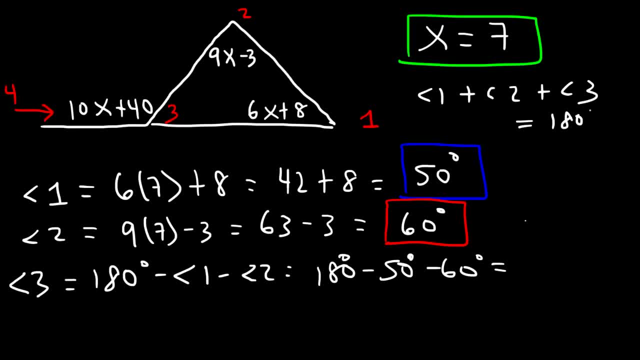 is greater, then blank is greater than blank. That is 얼마. And 1995 is the last angle, and pageld's length is 110, and thing simply means that angle 9 is the first of the three angles of the triangle. 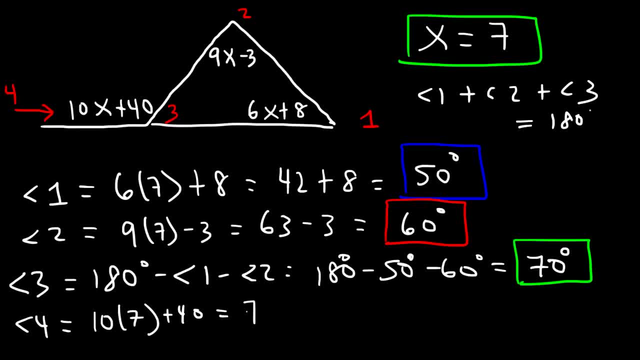 So angle 5, a true nominee, is equal to the η-sаюсь and 30. Ninety minus 50 minus yiz, minus 50 minus 60. So 180 minus 50 is 130. And 130 minus 60 is 70. So that's the value of angle 3.. Now angle 4 is 10x plus 40. So that's 10 times 7 plus 40. And 10 times 7 is 70, and 70 plus 40 is 110. And so we could see that is angle 5 is 180 and 30 is 40.. shutting on the замaric angle, Which is the angle 8, is 300, and so we can now calculate, while the angle 5 will be complementary. 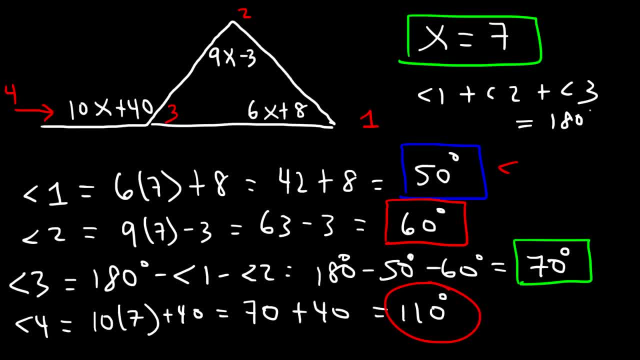 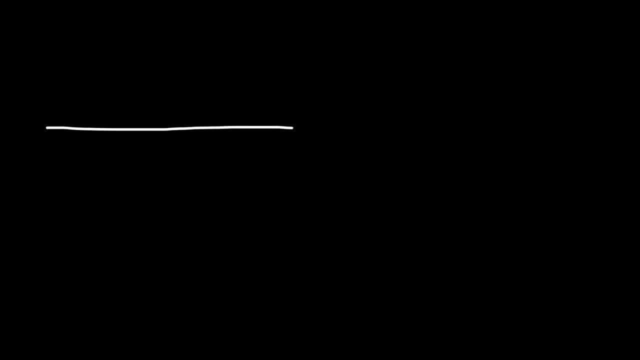 And so we can see that angle 4 is the sum of angle 1 and 2.. 50 plus 60 is 110.. Let's work on one more problem. So let's say: let's call this angle A, B, let's say this is C and this is D. 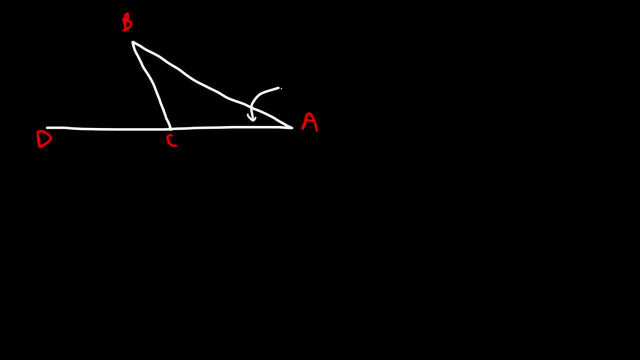 So angle A, we're going to say it's 8x plus 10.. And B, let's say it's x squared plus 5.. Let's say B, C, D is 16x. What is the measure of angle C? 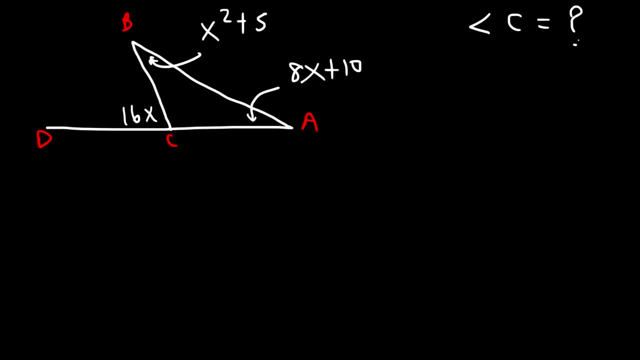 Go ahead and work on this problem. So before we can find the measure of angle C, we need to calculate the value of x. So using the exterior angle theorem, the exterior angle 16x is the sum of the remote interior angles, x squared plus 5 and 8x plus 10.. 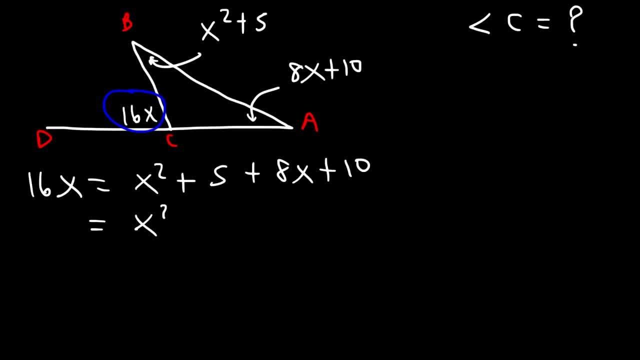 So let's combine like terms. On the right side, we have x squared plus 8x, And we can combine 5 and 10, which is 15.. Now all we need to do at this point is subtract both sides by 16, or 16x rather. 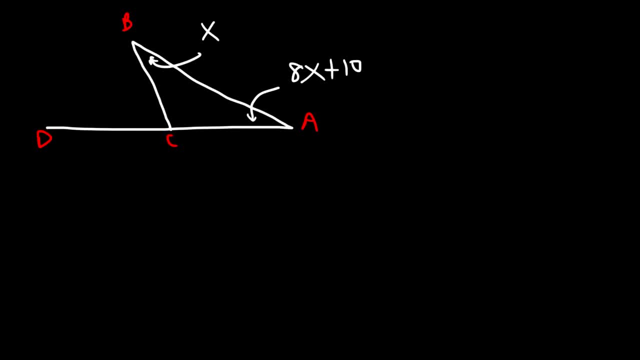 And B. let's say it's 8x plus 10.. And let's say it's x squared plus 5.. Let's say B, C, D is 16x. What is the measure of angle C? Go ahead and work on this problem. 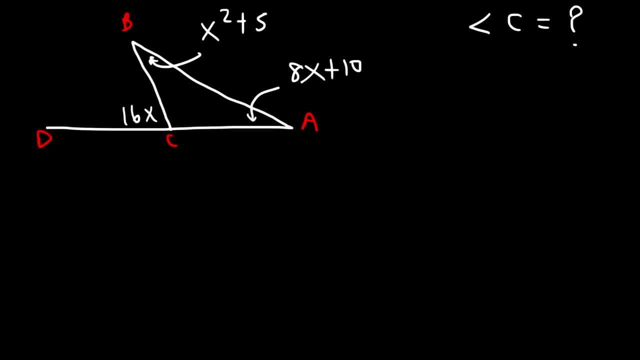 So before we can find the measure of angle C, we need to calculate the value of x. So using the exterior angle theorem. the exterior angle 16x is the sum of the remote interior angle. So we're going to calculate the value of x squared plus 5, and 8x plus 10.. 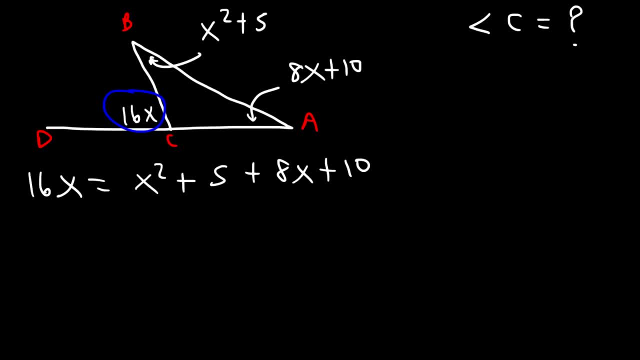 So let's combine like terms. On the right side, we have x squared plus 8x, and we can combine 5 and 10, which is 15.. Now all we need to do at this point is subtract both sides by 16, or 16x rather, and we could have a quadratic equation in standard form. 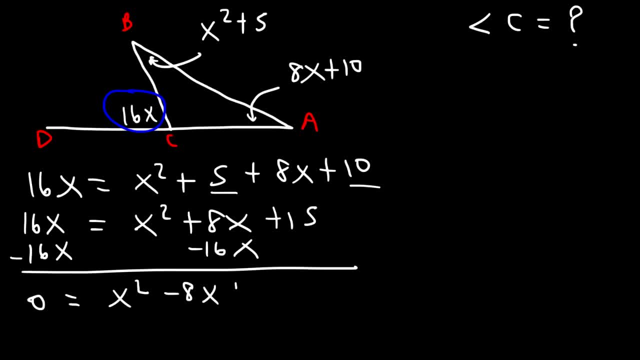 So 8x minus 16x is 16x. So 16x is negative 8x. So how can we solve this quadratic equation? In order to solve it we need to factor it. What two numbers multiply to the constant term 15, but add to the middle coefficient negative 8?? 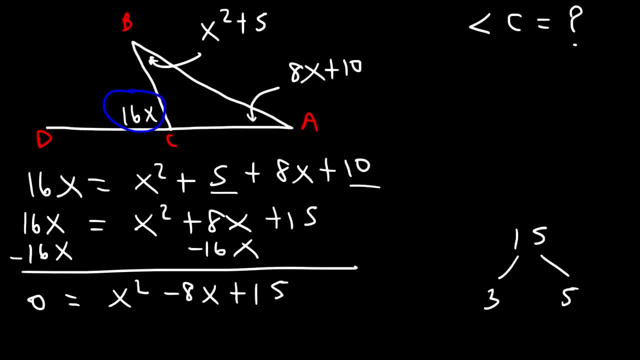 So there's two numbers that we need to worry about: 3 and 5.. 3 times 5 is 15.. 3 plus 5 is positive 8.. But we can make them both negative because they fit still multiply to positive 15.. So to factor it's going to be x minus 3 times x minus 5.. 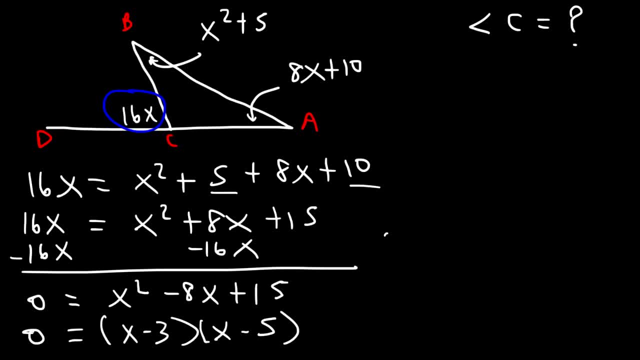 Now, at this point, you need to set each factor equal to 0. So x minus 3 equals 0 and x minus 5 is equal to 0. So if we add 3 to both sides, one possible answer that we could have is: x is equal. 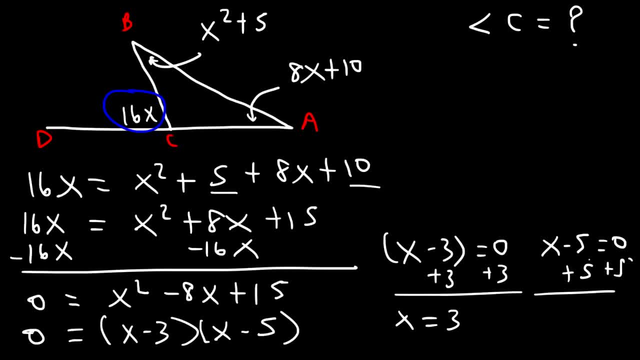 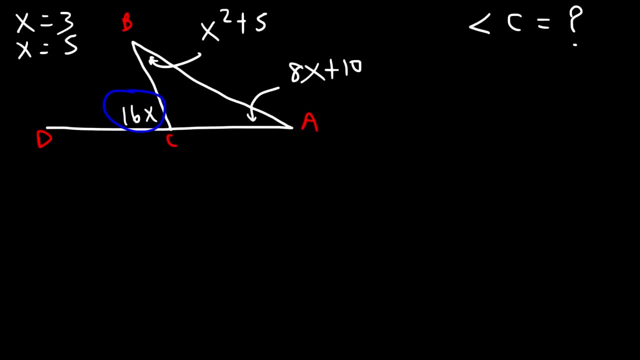 to 3.. And if we add 5 to both sides, the other possible answer is: x can equal 5.. So I'm just going to write that over here. So let's start with the first possible answer, if x is equal to 3.. 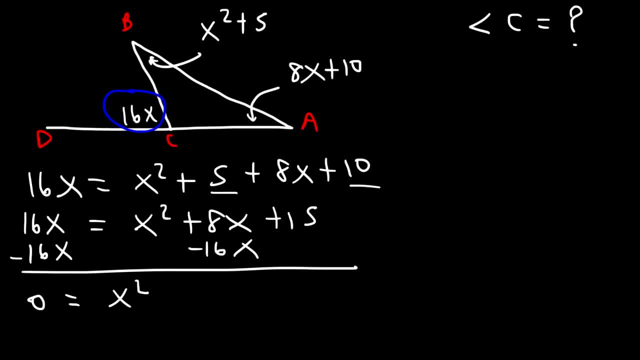 And we could have a quadratic equation in standard form. So 8x minus 16x is negative 8x. So how can we solve this quadratic equation? In order to solve it, we need to factor it. What two numbers multiply to the constant term 15,? 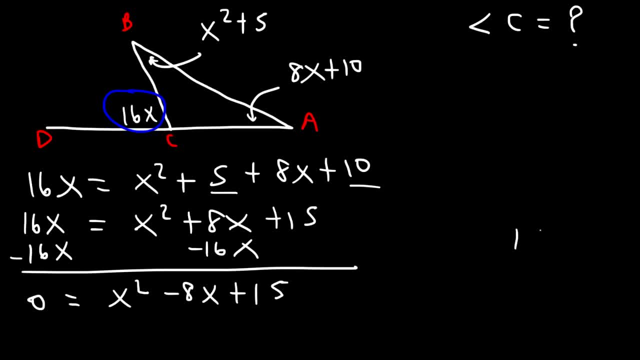 but add to the middle, We get the middle coefficient negative 8x. So there's two numbers that we need to worry about: 3 and 5.. 3 times 5 is 15.. 3 plus 5 is positive 8.. 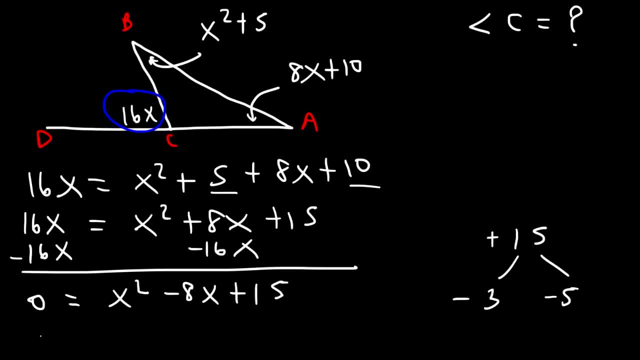 But we can make them both negative because they still multiply to positive 15.. So to factor it, it's going to be x minus 3 times x minus 5.. Now at this point you need to set each factor equal to 0.. 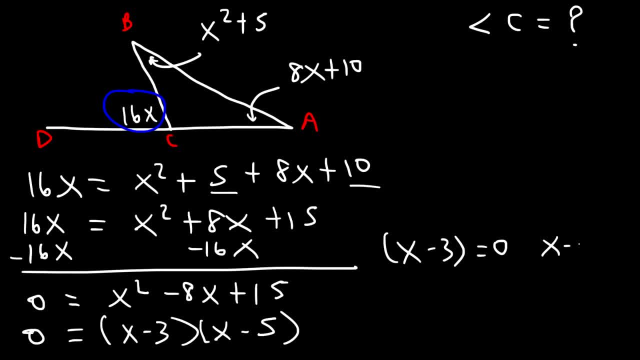 So x minus 3 equals 0, and x minus 5 is equal to 0.. So if we add 3 to both sides, one possible answer that we could have is x is equal to 3.. And if we add 5 to both sides, the other possible answer is x can equal 5.. 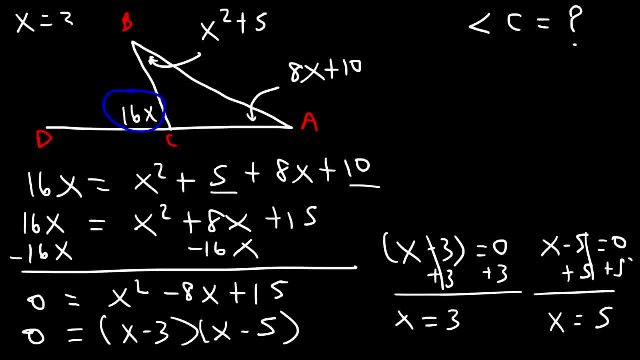 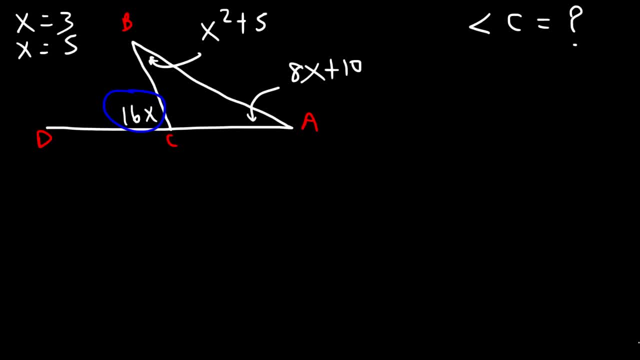 So I'm just going to write that over here. So let's start with the first possible answer. if x is equal to 3.. So angle C is going to be 16.. It's going to be 16 times 3,, which is 48.. 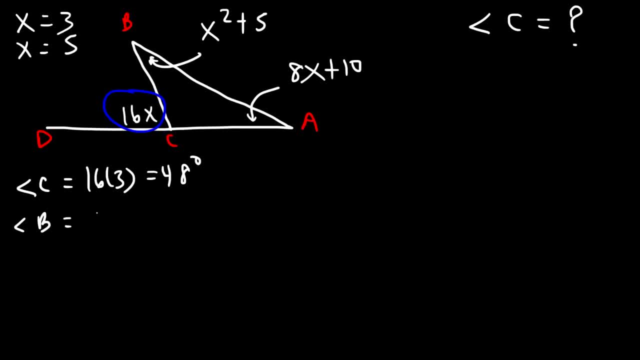 And angle B is going to be 3 squared plus 5.. 3 squared is 9 plus 5.. That's 14.. Angle A is going to be 8 times 3 plus 10.. 8 times 3 is 24.. 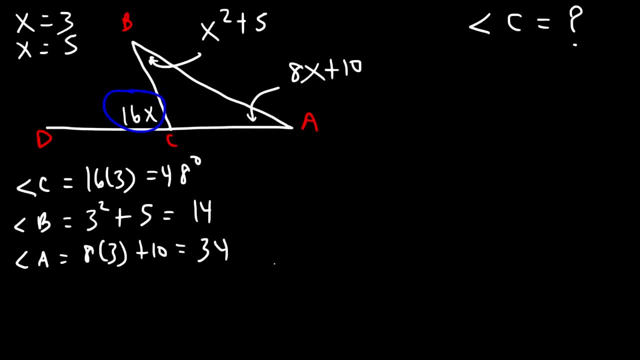 24 plus 10 is 34.. And so, And then angle C is basically: Well, angle C and angle the 16x angle they have to add up to 180.. So we can say that angle C is 180 minus 16x or minus 48.. 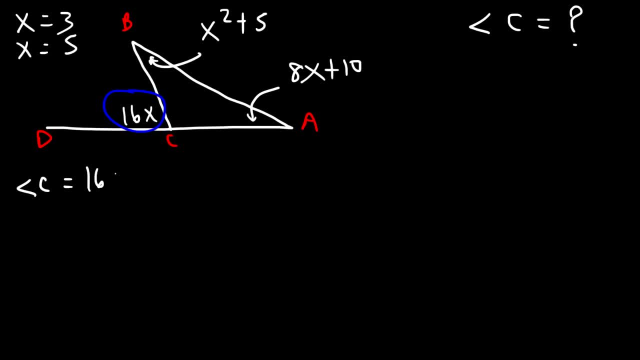 So angle c is going to be 16 times 3, which is 48.. And angle b is going to be 3 squared plus 5.. 3 squared is 9 plus 5, that's 14.. Angle a is going to be: 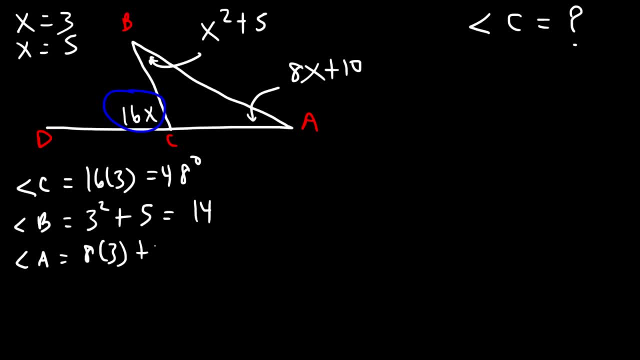 8 times 3 plus 10.. 8 times 3 is 24.. 24 plus 10 is 34.. And so, and then angle c is basically well, angle c and angle, the 16x angle, are going to be 8 times 3 plus 10.. And so, and then angle c is basically well, angle c is going to be. 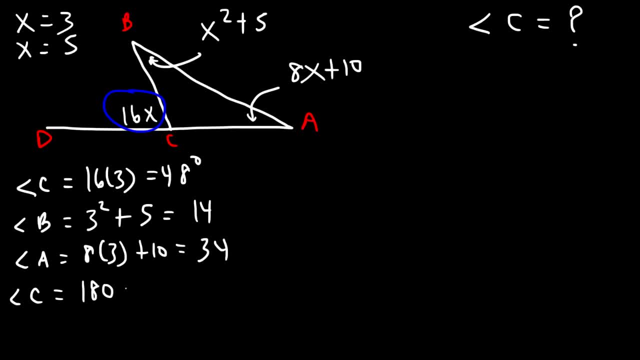 They have to add up to an 80. So we can say that angle c is 180 minus 16x or minus 48. I need to distinguish these two angles, So let me adjust their names, because they can't both be angle c. 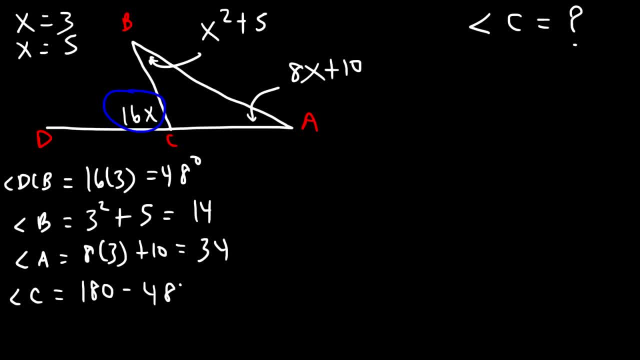 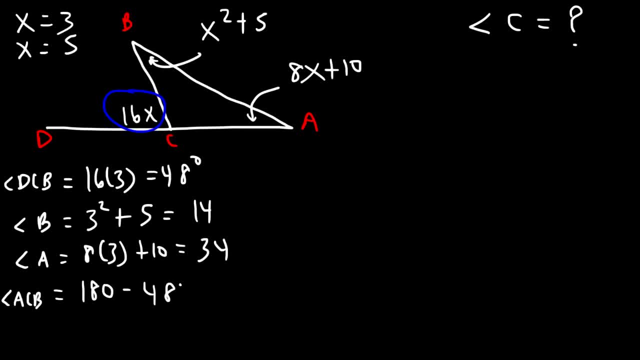 And that is angle acb. So acb, this angle, that's 180 minus 48.. Which is 132.. And so one possible answer for the value of c, which I specify, which c this is meaning: bca or acb. 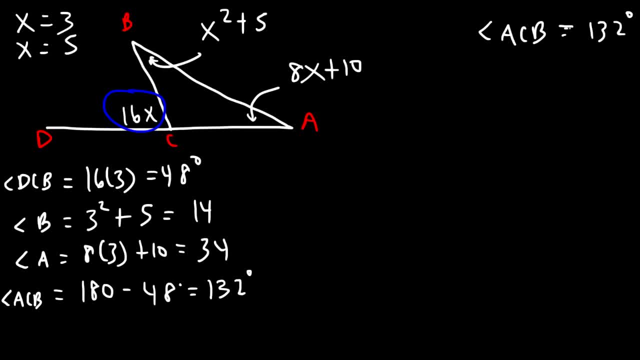 is 132 degrees. now let's calculate the other possible angle. so if X is equal to 5, so DCB, this angle, that's going to be 16 times 5, which is 80. and then we have angle B, which is x squared plus 5, so that's going to be 5 squared plus 5, 5. 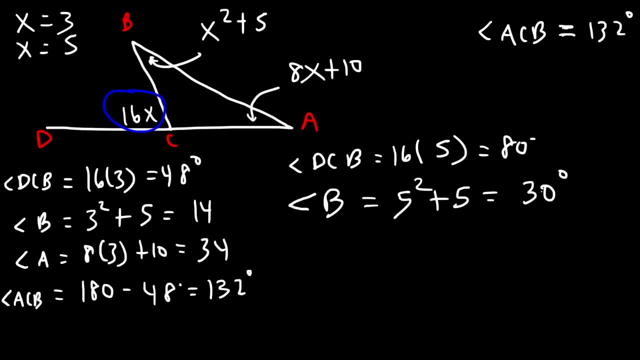 squared is 25 plus 5, that's 30 degrees. and then angle a 8x plus 10, or 8 times 5 plus 10, so that's going to be 40 plus 10, so 50 degrees and then finally ACB. 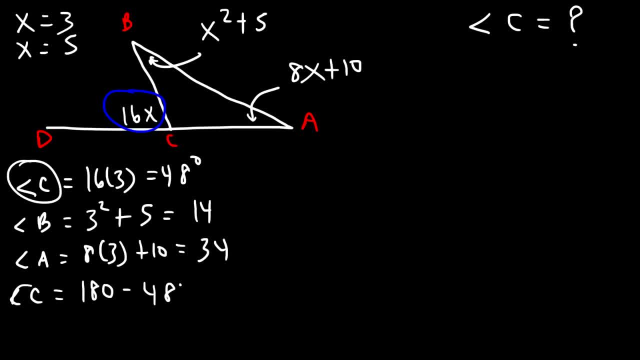 I need to distinguish these two angles, So let me adjust their names, because they can't both be angle C, So this is going to be angle. So this is going to be angle DCB And this is the angle that we're looking for. 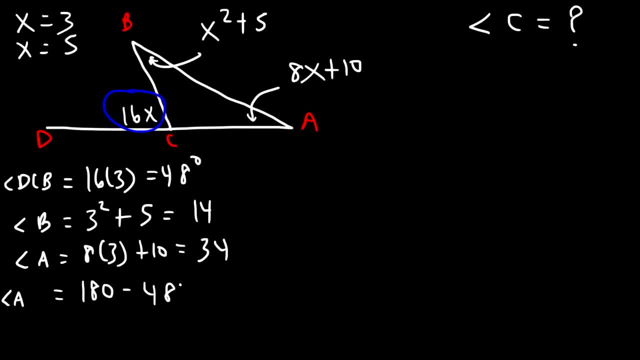 And that is angle ACB. So ACB, this angle, that's 180 minus 48.. Which is 132.. And so One possible answer for the value of C, Which I specify, which C this is Meaning: B, CA or ACB. 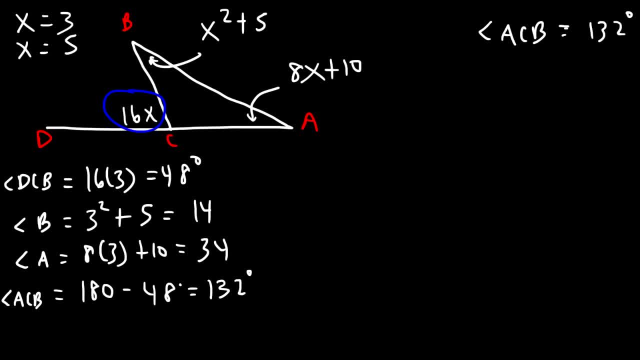 Is 132 degrees. Now let's calculate the other possible angle. So if X is equal to 5.. So DCB, this angle, that's going to be 16 times 5., Which is 80.. And then we have angle B. 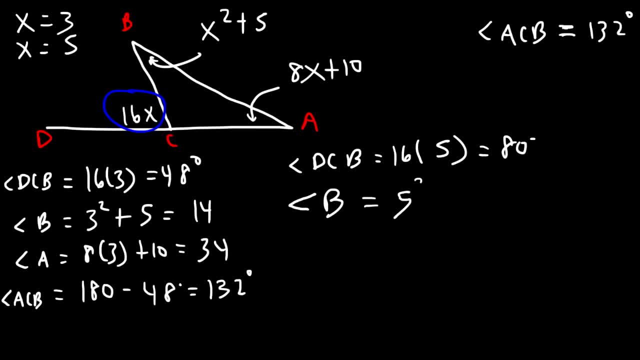 Which is X squared plus 5.. So that's going to be 5 squared plus 5.. 5 squared is 25 plus 5.. That's 30 degrees. And then angle A 8x plus 10, or 8 times 5 plus 10.. 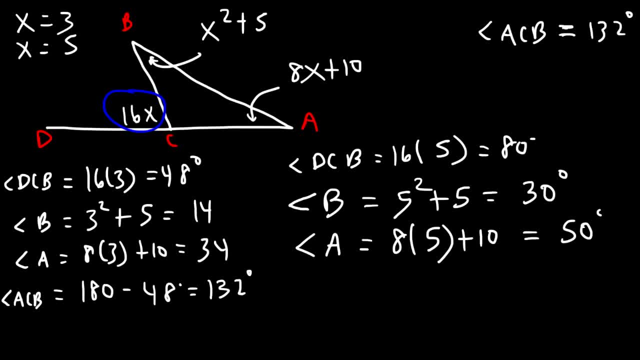 So that's going to be 40 plus 10.. So 50 degrees. And then finally ACB, That's 180 minus DCB, So minus 80.. Which will give us 100.. So we have two possible answers: It could be 132 or it could be 100. 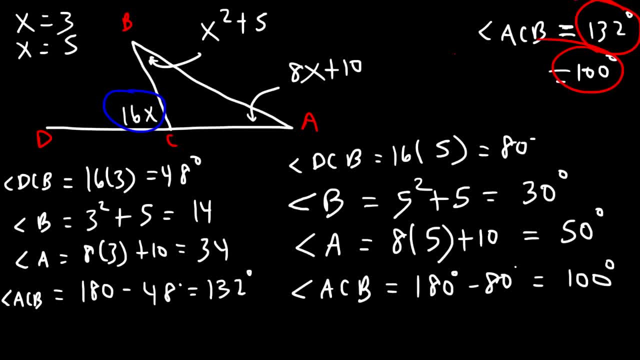 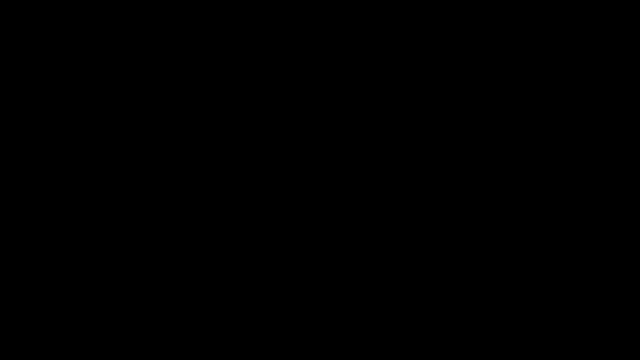 And so we're going to stop here. So that's it for the exterior angle theorem. So now you know what it is, And now you know how to use it to solve missing angles and calculating the value of X. Thanks for watching. See you next time.